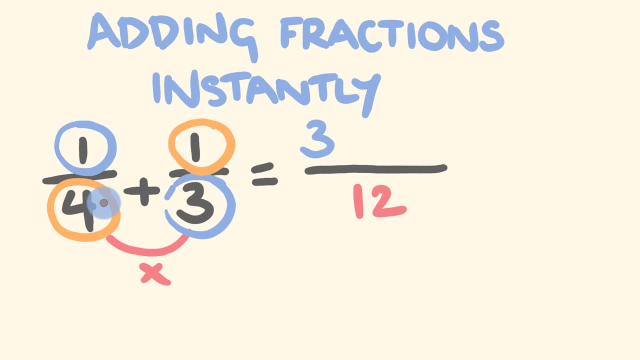 by this number at the top right here. Okay, so one times four is equal to four, and because we're adding, let's put the addition symbol there. So what have we got? We have the following: three plus four is equal to seven. The bottom number, the denominator, is 12, and there's our answer, As you. 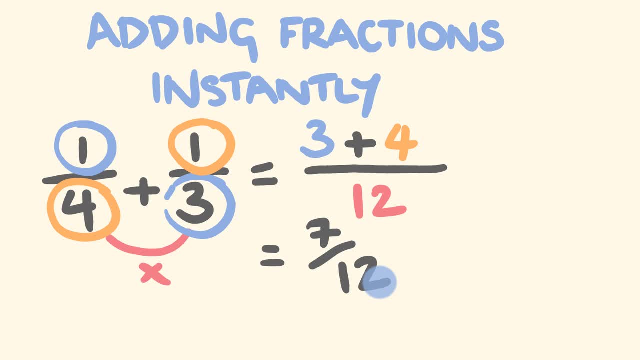 can see, there's not tons of working out, working out common denominators. We've pretty much just done this directly. So what about another example? Okay, what about we do this one? What about we do two thirds? and to this we're going to add three fifths. Okay, a bit harder. 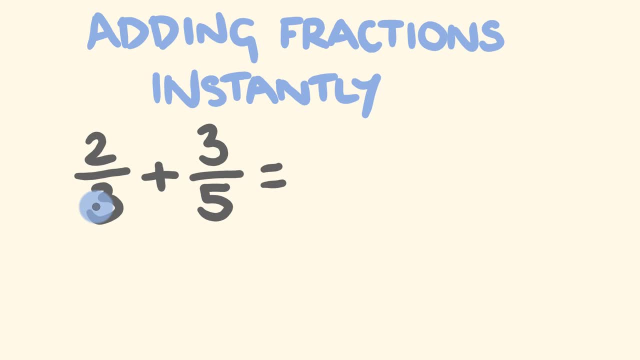 now a bit bigger, and I can tell you that our answer is going to be over one, So we are going to have to simplify it at the end, and occasionally you will have to do that. So first off, let's get our answers here. Three times five is equal to fifteen. 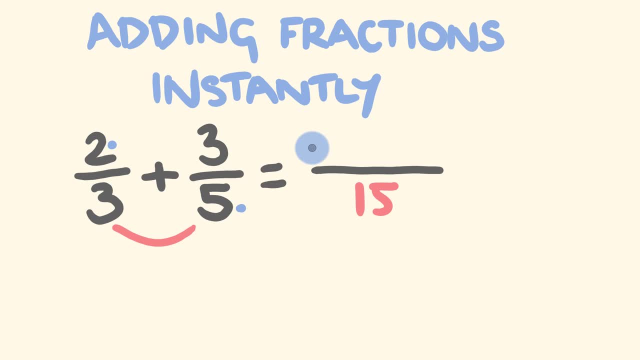 We're going to multiply this by this: two times five is equal to ten. The next one, three times three, is equal to nine, and we're going to add our answers. We're adding fractions here. So ten plus nine is equal to nineteen over fifteen. Now we can simplify this further. We've got an improper fraction. 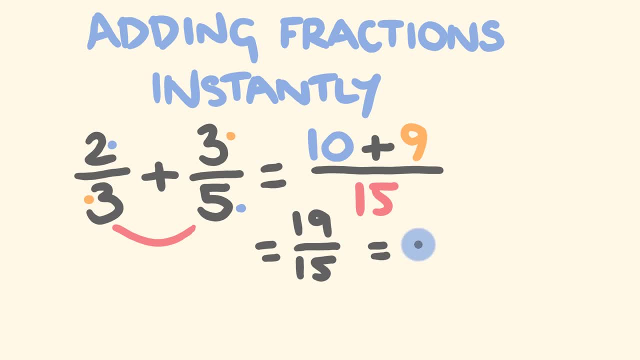 answer here. but let's simplify it now. Nineteen divided by fifteen is equal to one, and there is, the four goes there, and our bottom denominator here goes here. Okay, so one and four, fifteenths, All right. one more example then I'm going to give a bunch of them to you to do. Okay for our third. 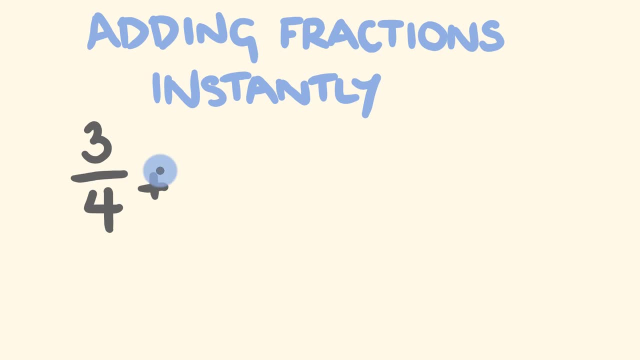 example, let's get three quarters and to this let's add three over seven. I'm going to give you a bunch of these to do in a second. We'll just get through this example. We have this line here and let's work out our denominator. Four times seven is twenty eight. 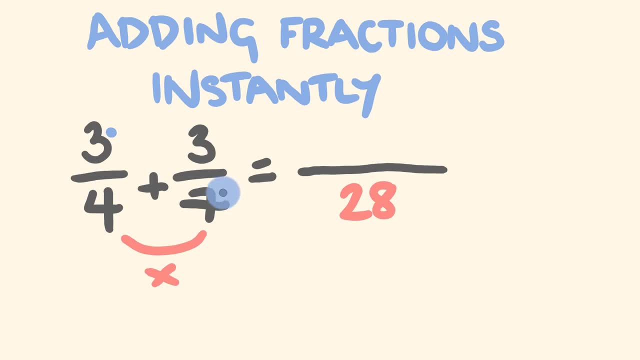 Let's work out: top left times the bottom right: Three times seven is equal to twenty one. Three times four is equal to twelve, and we are adding here. so 21 plus 12 is 33.. 33 over 28.. What does this equal? Well, we can simplify this a bit further now. 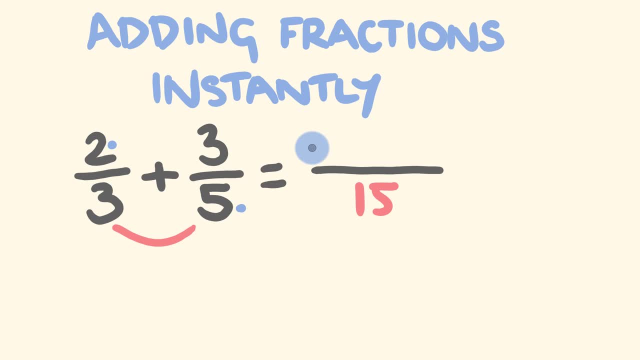 We're going to multiply this by this: two times five is equal to ten. The next one, three times three, is equal to nine, and we're going to add our answers. We're adding fractions here. So ten plus nine is equal to nineteen over fifteen. Now we can simplify this further. We've got an improper fraction. 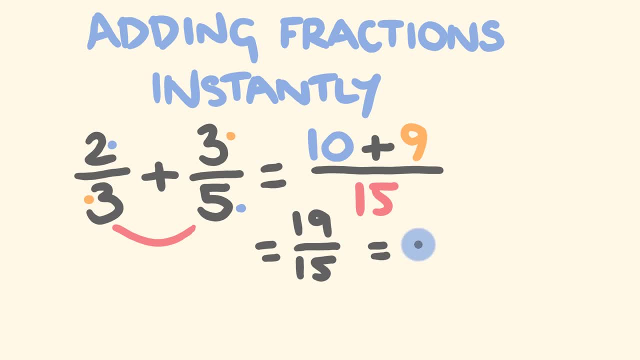 answer here. but let's simplify it now. Nineteen divided by fifteen is equal to one, and there is, the four goes there, and our bottom denominator here goes here. Okay, so one and four, fifteenths, All right. one more example then I'm going to give a bunch of them to you to do. Okay for our third. 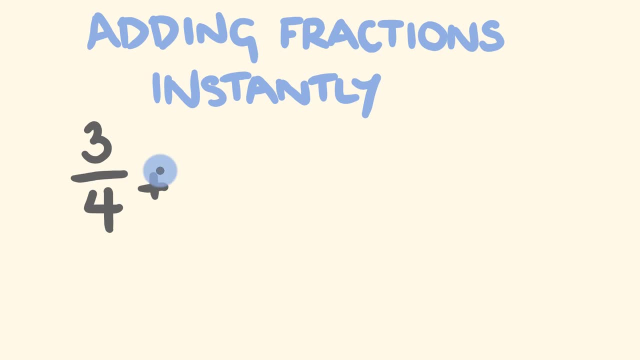 example, let's get three quarters and to this let's add three over seven. I'm going to give you a bunch of these to do in a second. We'll just get through this example. We have this line here and let's work out our denominator. Four times seven is twenty eight. 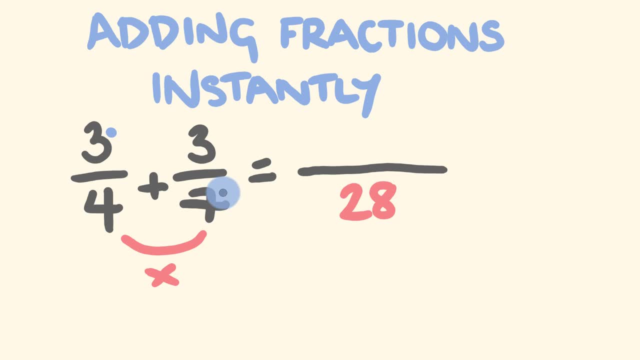 Let's work out top left times the bottom right. Three times seven is equal to twenty-one. Three times four is equal to twelve, and we are adding here. So twenty-one plus twelve is thirty-three, Thirty-three over twenty-eight. What does this equal? Well, we can simplify this a bit. 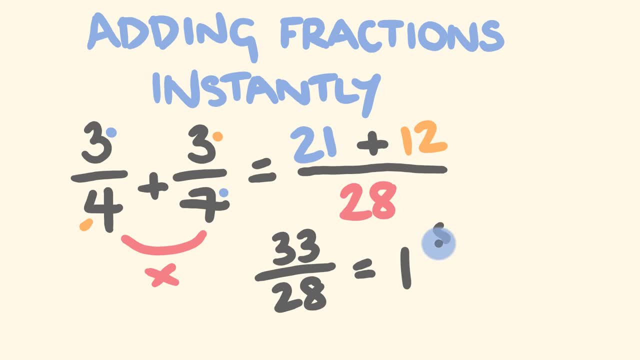 further. now. Thirty-three divided by twenty-eight is one and there is five left over Five. it's going over 28 anyway. what about a few examples for you to do? okay, what about we go uh one quarter, and to this we're going to add uh three over five. you can do that one and we're also going to do. 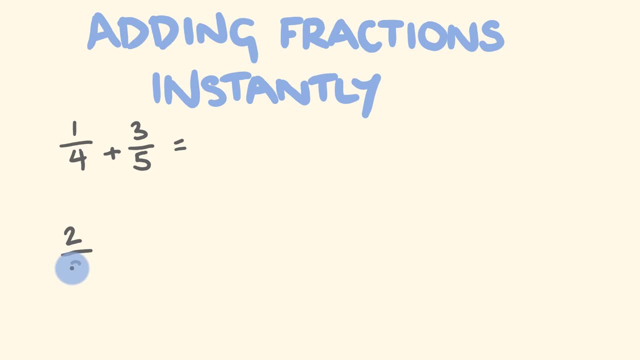 uh, two over nine, and to this we're going to add uh one over four a quarter. let's see what our answers are. so first off, let's work this out, okay, uh, four times five is equal to 20, all right. next we have one times five, and this is equal to five. we have this one here three times.